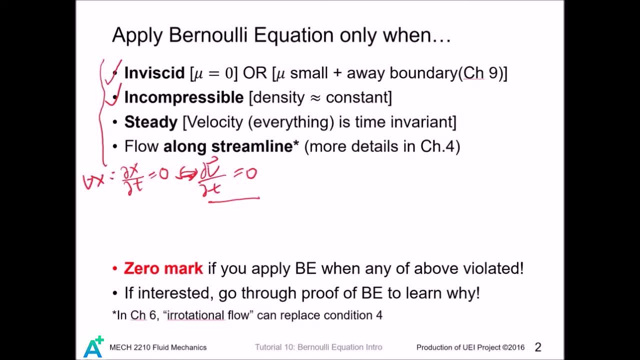 It does not necessarily mean that the particle does not change with time. It does not necessarily mean that the particle does not accelerate. It is because acceleration can still be a function of position. We shall cover it later in this video And there is an example about that. So we are done. 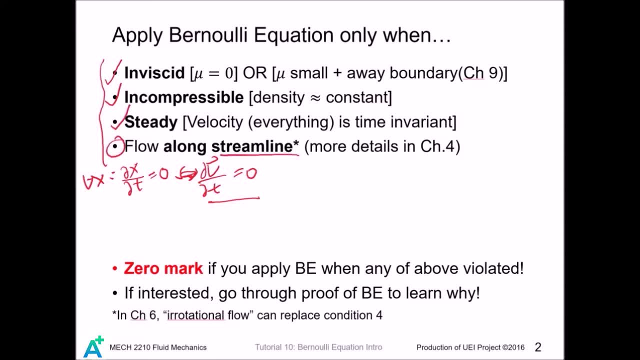 with this one. For the last one, what is streamline? Streamlines by definition aligns tangential to the velocity field. So if we have a velocity field, go this way, then we have these two streamlines. We are going to work on that in the next chapter. Under steady conditions, streamlines are just. 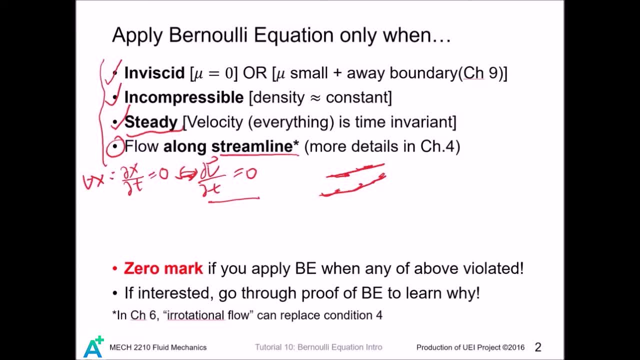 trajectories of the particles or pathlines. Imagine we have a particle here. If the flow is steady, this guy will go here after some period of time. So I repeat, you must make sure that these four conditions are satisfied before applying Bologna equation. Professor Li told. 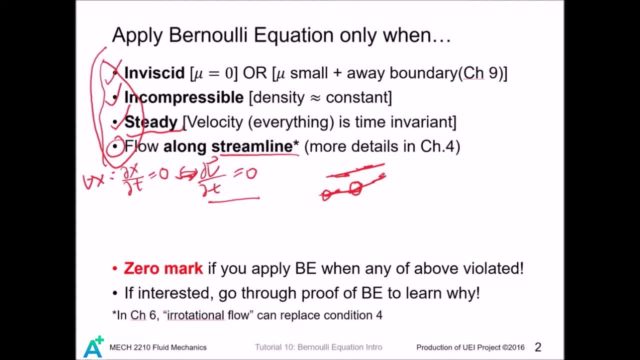 us that we would obtain zero mark in the midterm if we abuse Bologna equation last year. If you are really interested in knowing why these conditions must be satisfied in applying Bologna equation, you shall go to lecture and derive Bologna equation once yourself. 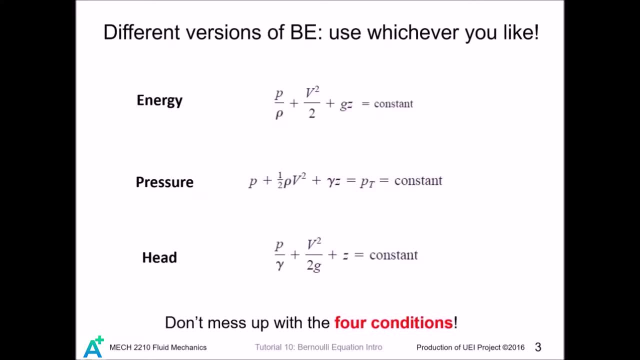 There are three forms of Bologna equation, and you may use whichever convenient to the problem. In fact, I have talked about the first form in the tutorial 2 already. The first term here measures the flow work, The second term is the kinetic energy And the last one is gravitational. 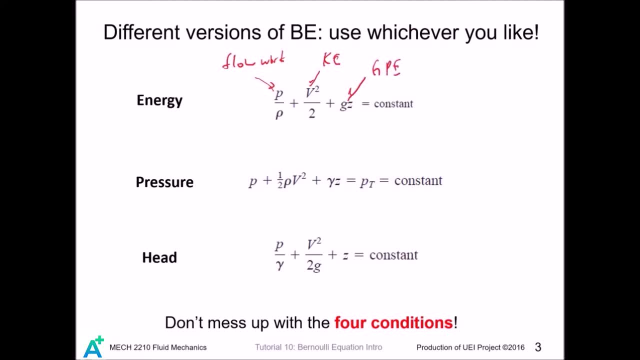 potential energy. Although the book uses Newton's second law to derive the formula, the Bologna equation can be thought as energy balance If we multiply the first one by the density and we get the second one. So each term here has the same unit as pressure People call the first. 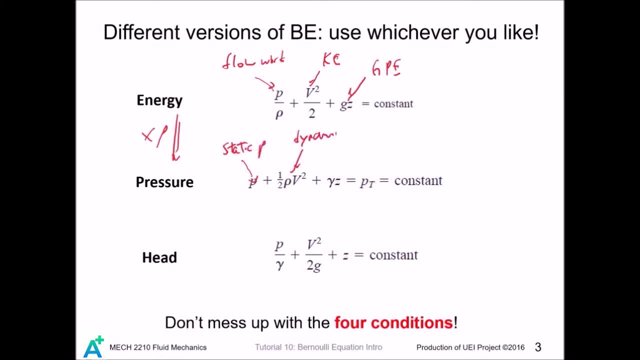 one as static pressure, the second one as dynamic pressure and the third one as elevation pressure, And people call this sum as total pressure. But I have one thing more to talk about this version: If the flow is horizontal, then the elevation pressure goes away. 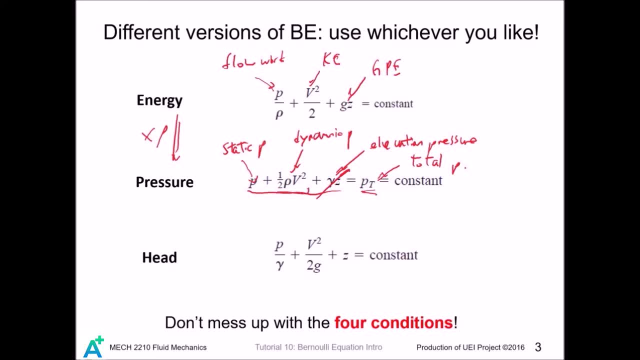 Then the total pressure is just the sum of these two terms. Then points with the zero velocity has the highest pressure In fluid mechanics. points with zero velocity are called stagnation points And their pressure are called stagnation pressure. That pressure is simply the total pressure And it can be evaluated by using some of these two. 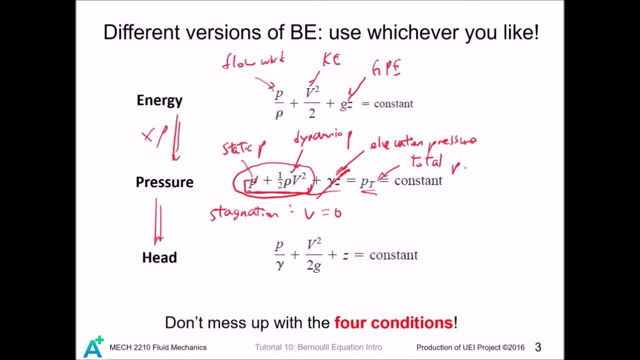 terms at every point. Finally, if we divide the second one by the specific weight, we get the third one, And now each term here has the unit of length. People call the first one as pressure head, one as Curiosity hat and the last one as Elevation hat. 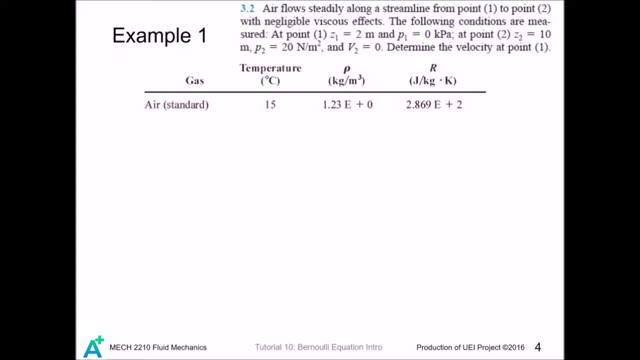 We now do a quick example to illustrate how to use Boulogne equation. Before applying Boulogne equation we must ensure that all the four conditions for Boulogne equation is satisfied. First, we have negatible viscous effect and we have steady and also we have a long stream. 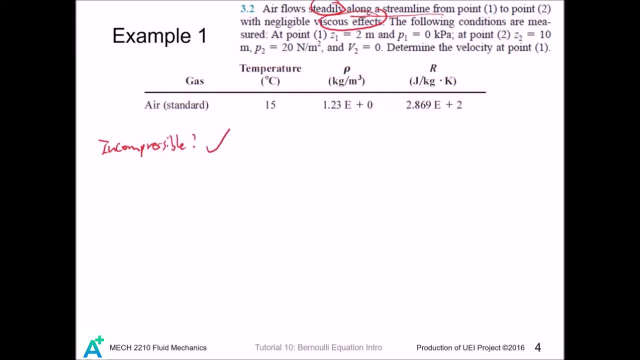 line. But what about incompressible? And we just say this one is okay because the change in pressure is just 20 Pascal. We will further justify for that in the last part of the video. So we now write down the Boulogne equation, and that means for points 1 and 2, and we 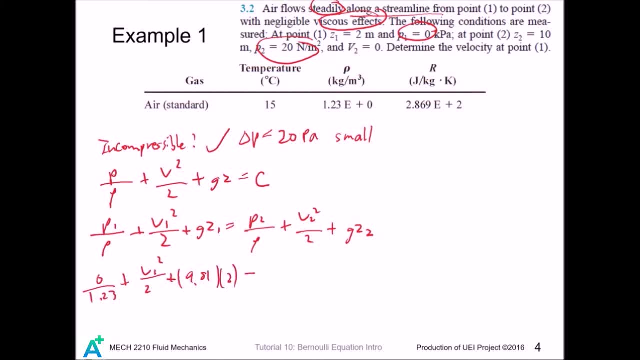 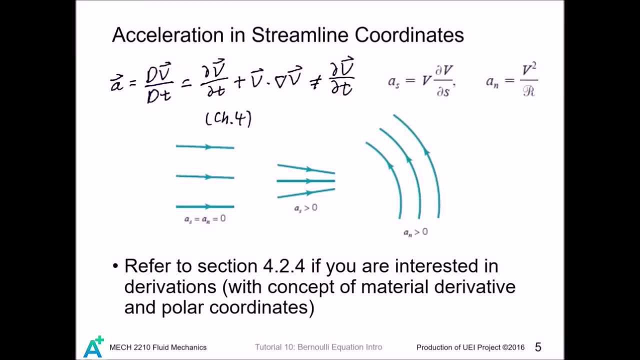 substitute in the values. So we have, And we call it Boulogne: Continue to solve for v1, and we are done with this easy example. As I said previously, as you are going to learn in chapter 4,, acceleration is the material. 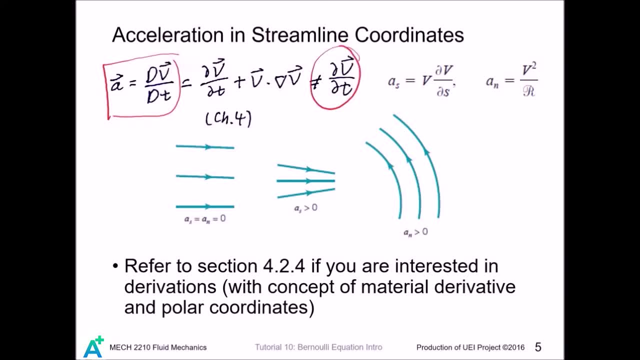 derivative of velocity and that is not equal to partial v, partial t- Even if this term is gone, you still have this term- and in streamline coordinates, under steady conditions, the streamline component and the normal component of accelerations are given here. 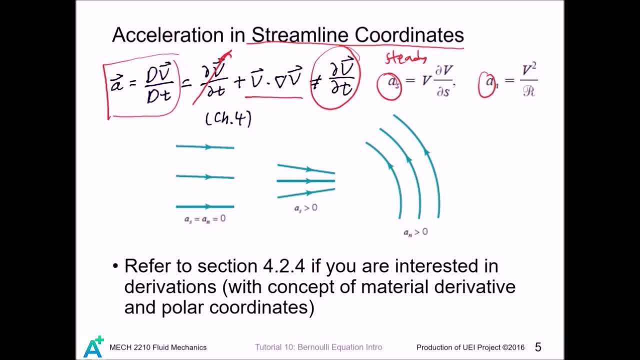 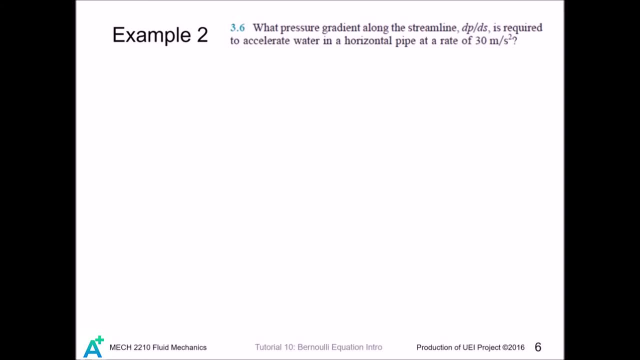 And this figure below shows that In fact the Boulogne equation can be manipulated to obtain information about streamline component of acceleration. We now do a quick example about that. So we have water here, Water can be assumed as incompressible and we further assume that the flow is steady. 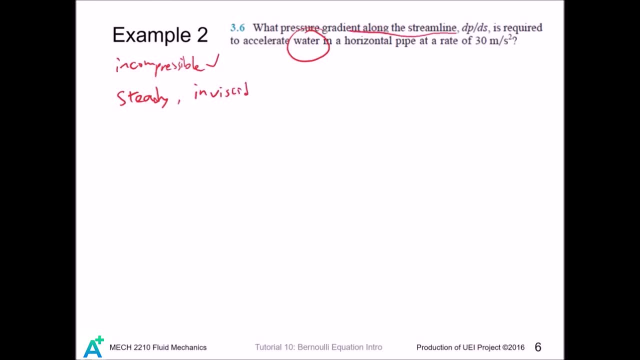 and all viscous effect can be neglected. Now it's a long streamline, so all the assumptions have been fulfilled. but Boulogne equation: we write down And we substitute And we differentiate it with respect to the streamline variable. Now the pipe is horizontal, so this just go away. 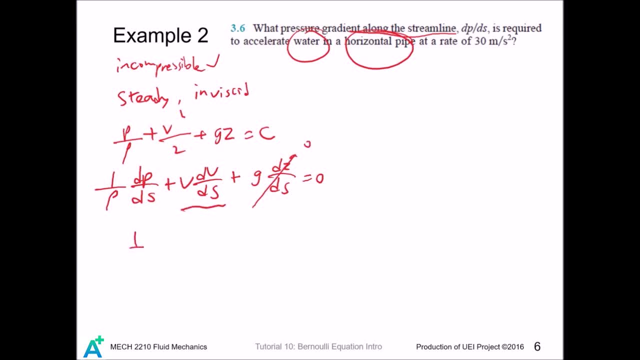 And this term is the streamline component of acceleration. So we write down, So we have, And this is the pressure gradient required to accelerate the fluid. Now for interest, In fact for compressible flow, We could use a weaker version of Boulogne equation. 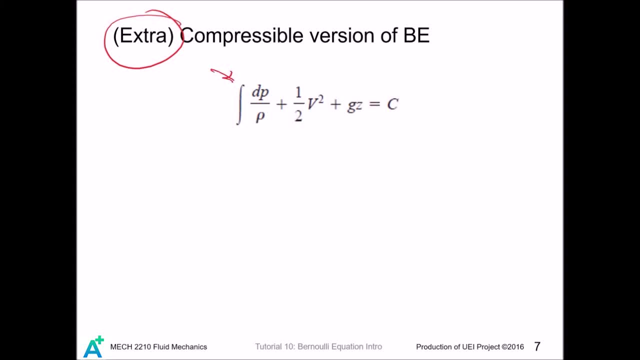 This equation is also true for compressible flow. To see why you have to go through the definition of Boulogne equation For gases. we have the ideal gas law, So this term equals And that is, And we integrate. So we conclude that the gas version of Boulogne equation is just 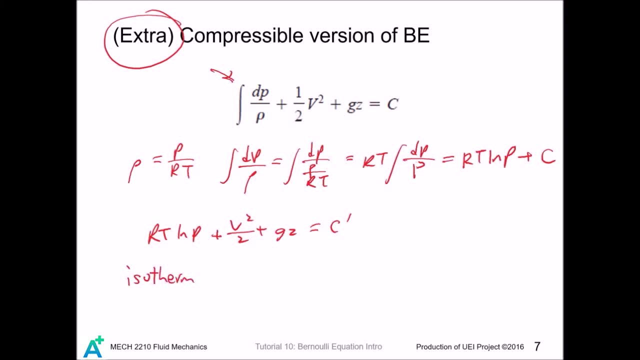 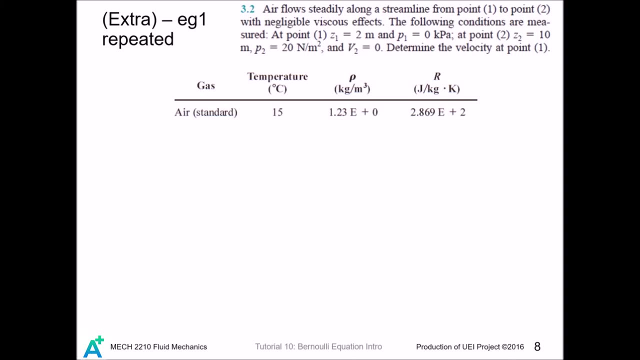 This formula is just true for isothermal process. Now we see why the incompressible assumption is appropriate here in the first example. First we compare the density From the ideal gas law. we have P directly proportional to the density. So the density exposed to is 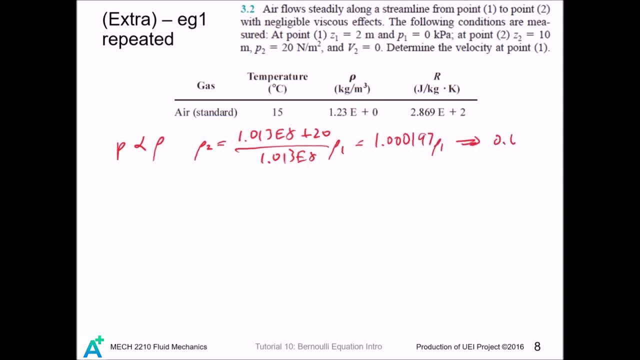 And that is. That is just a small difference And from the previous formula We have, We assume this process is isothermal And we continue to write down a formula And we substitute in a values And solving for three one, we get the same answer. 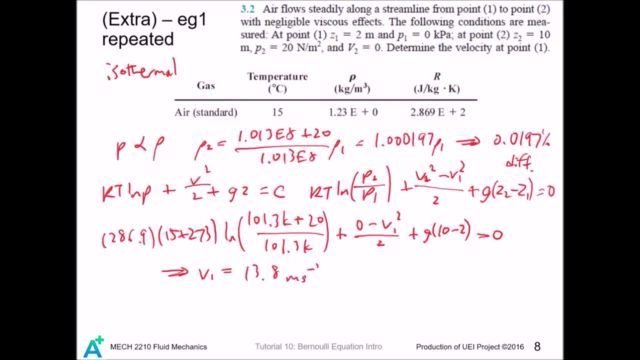 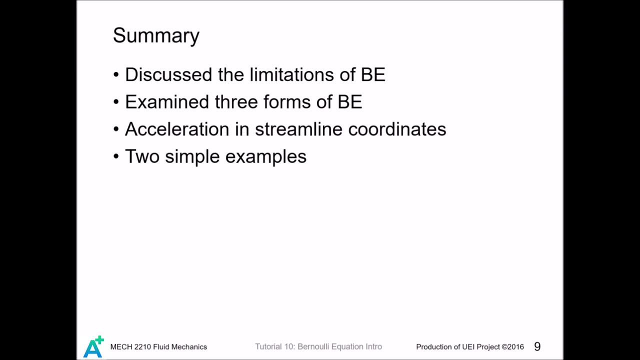 And we could do this: the same answer. if such a small difference in density, the answer is just the same with the two different versions of baloney equation. in summary, today we discussed the limitations of baloney equations. we look at the three forms of baloney equation and we also look at the concept. 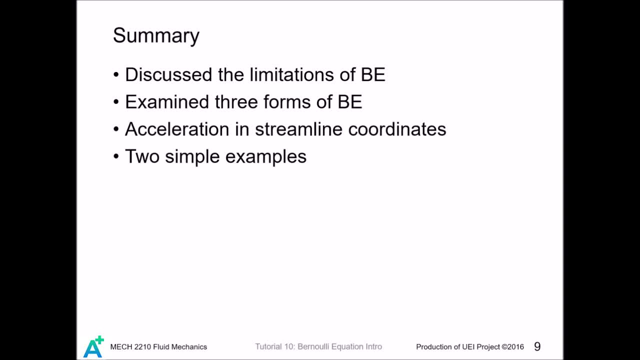 of acceleration along streamline. we also work through two examples about that. hope you enjoy today's tutorial and thanks for watching. feel free to ask us any questions and give us any feedback in the comments.